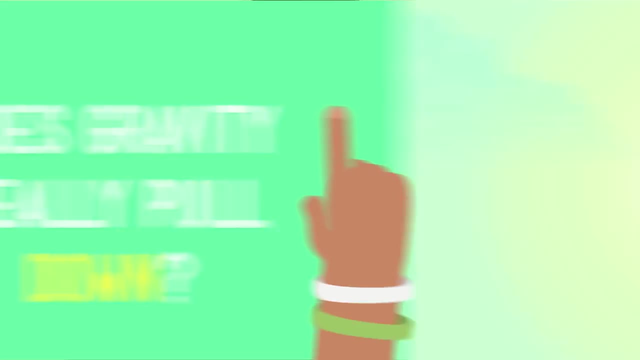 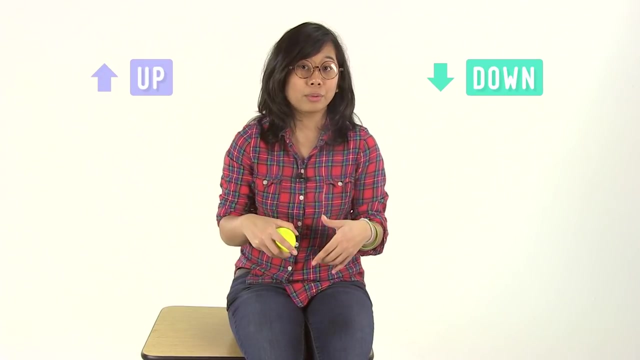 I mean, does gravity really pull down? When we talk about gravity and we say things like up or down, we don't mean those things in the sense that you're used to. In this case, up just means away from the Earth, and 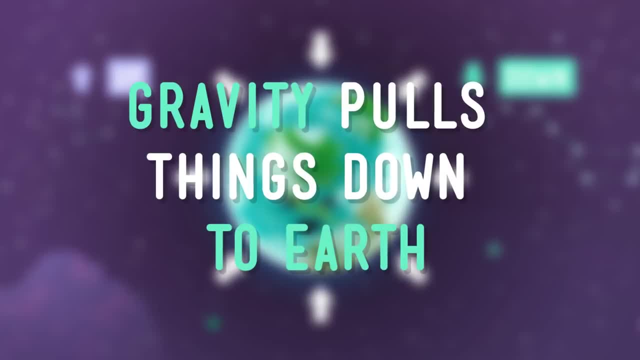 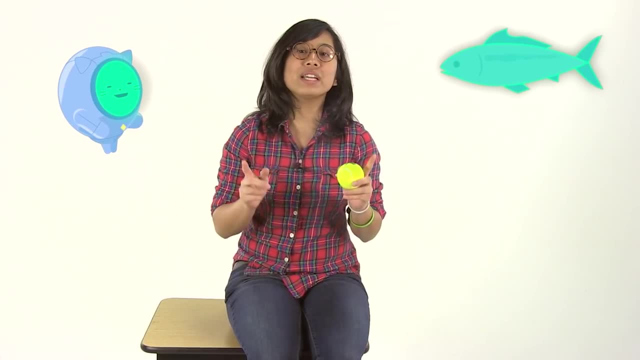 down means toward it. So when you hear people say gravity pulls things down to Earth, they really mean that gravity pulls things toward the Earth. Now think of it this way: Gravity is the force of attraction between any two objects made of matter. right, Well, I have. 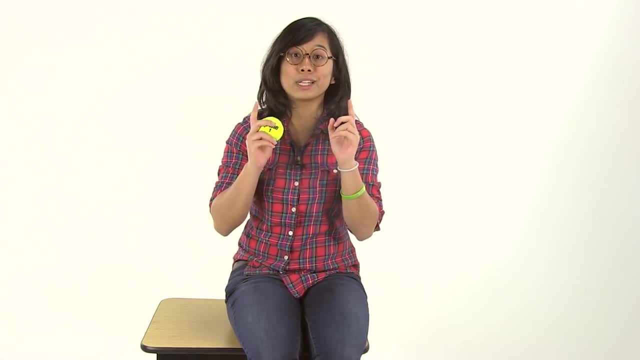 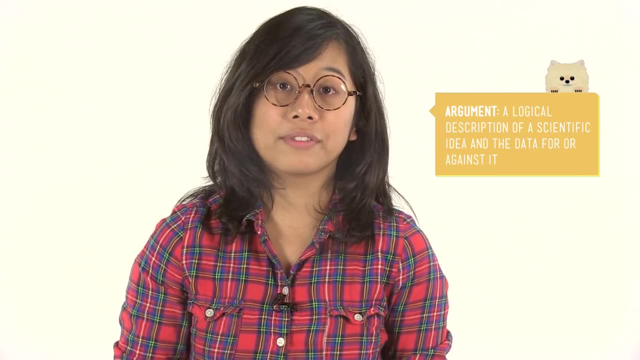 news for you: You're made of matter, and so is the Earth. That means you and the Earth have an attraction to each other. Aww you guys. Anyway, the scientific argument for gravity is that any object that's on or close to Earth's 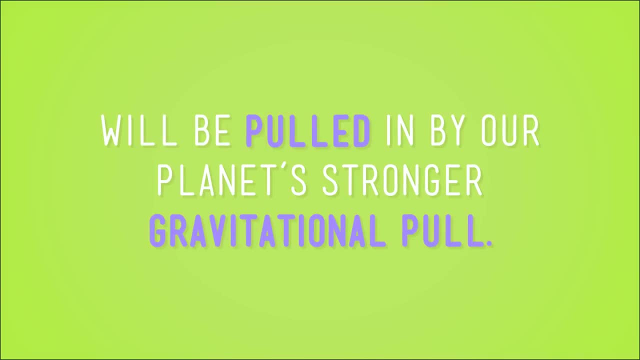 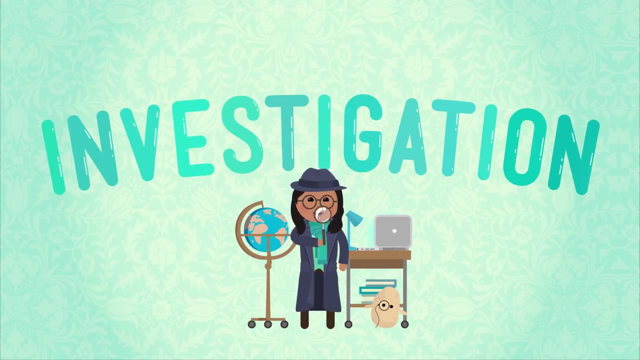 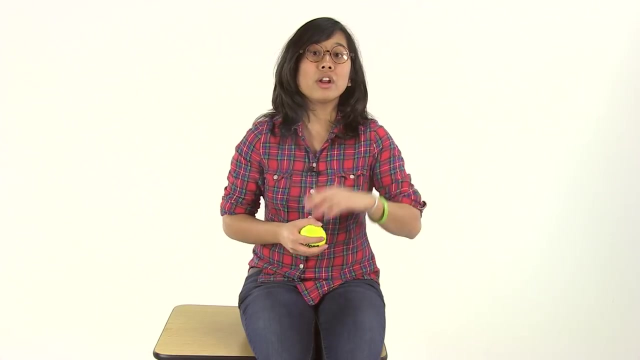 surface and is made of less matter than Earth, will be pulled in by our planet's stronger gravitational pull. Want to do a little demonstration To show how Earth's gravity can pull an object like the penguin we mentioned before toward it, no matter where on Earth that penguin is. all you need is a tennis ball and a rubber. 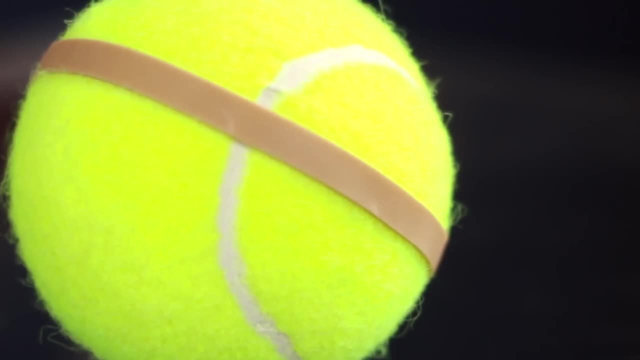 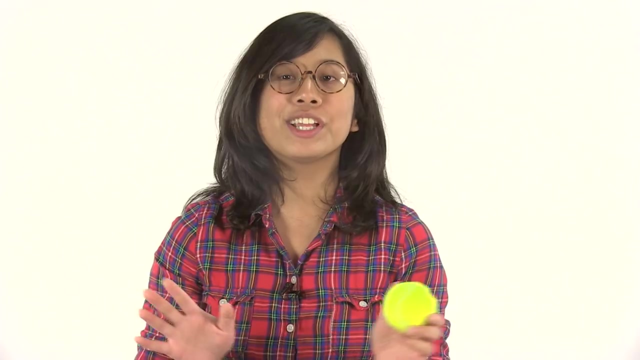 band. Oh, and your index finger. Now let's pretend the tennis ball is Earth and the rubber band represents the force of gravity That makes your finger our adorable little penguin just chilling on the surface of the Earth. Now stretch the rubber band around. 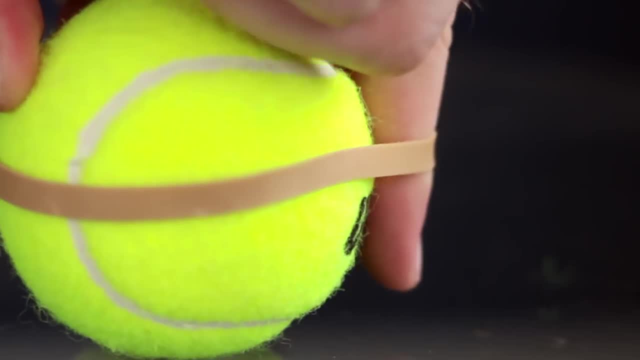 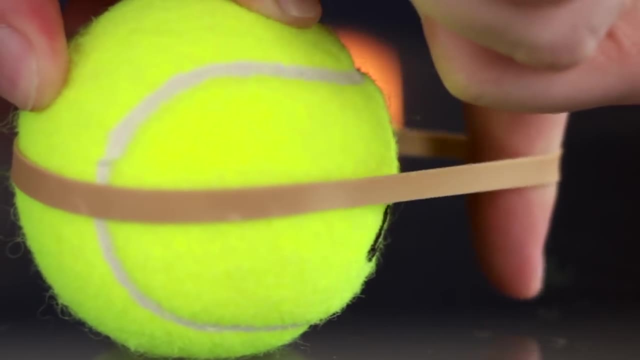 your tennis ball Earth and stick your finger under the rubber band. Now try to lightly pull your finger away from the ball. The penguin is trying to jump off the Earth, even though penguins can't fly. What are you doing, penguin? 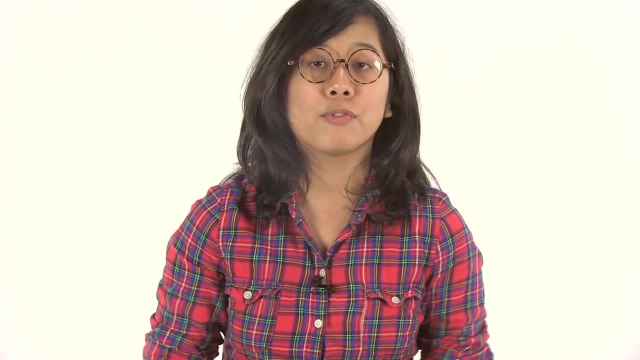 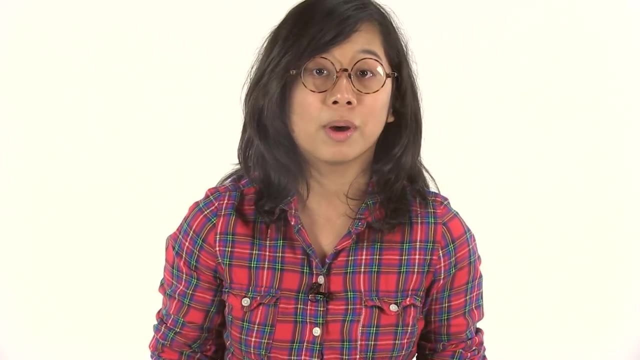 But what happens? Not much. Your finger doesn't get far before the rubber band pulls it back toward the ball right, And the effect is the same, no matter where your finger penguin is on your Earth ball, Whether it's at the top or the side or on the very bottom. the 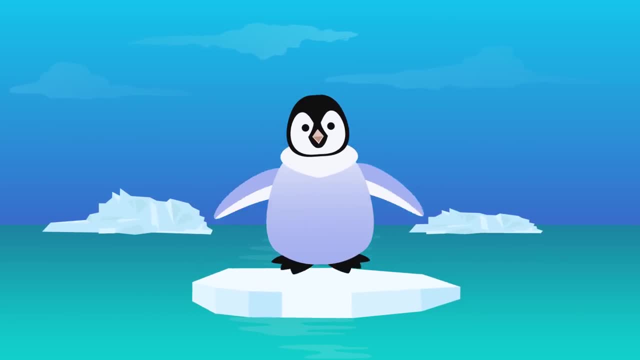 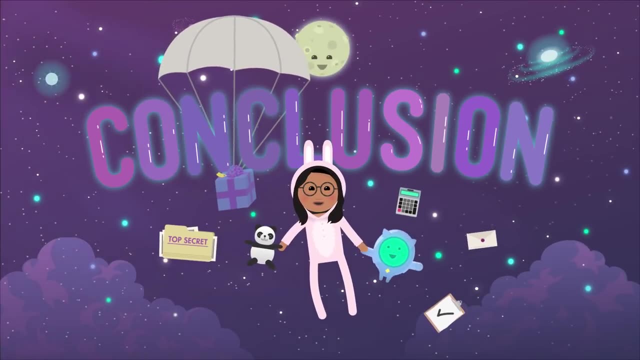 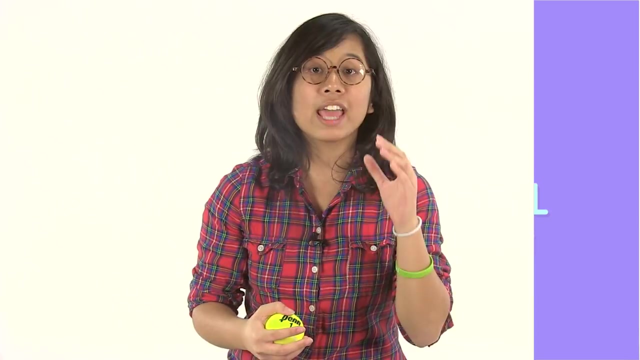 same thing happens: The penguin is forced back to Earth, no matter how hard it tries to jump off. So what does this mean? It means that no matter where on Earth an object is, the planet's gravitational pull will draw the object toward it, And that's how you should think about gravity. It's the